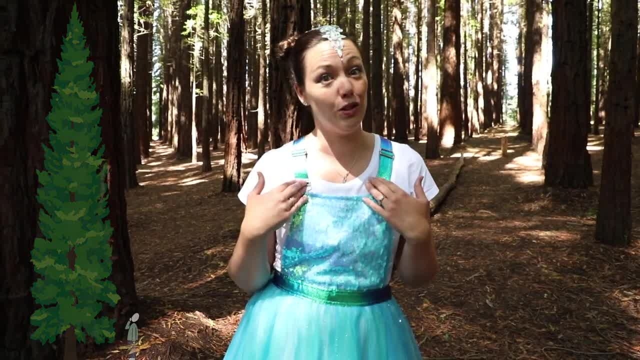 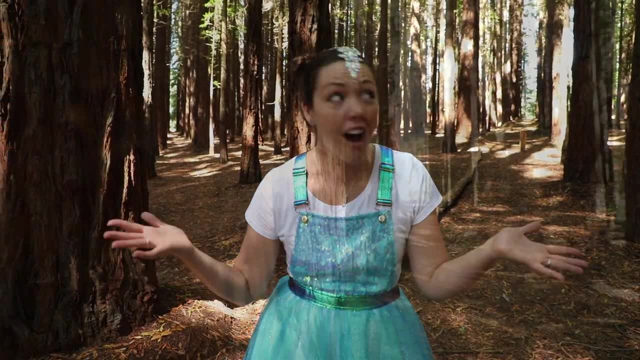 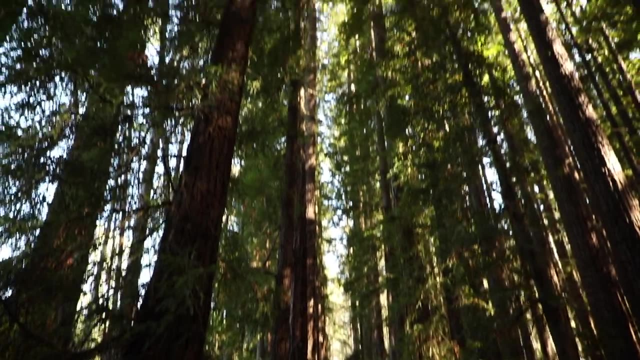 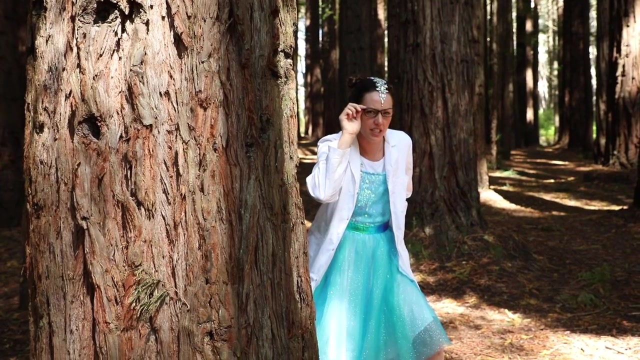 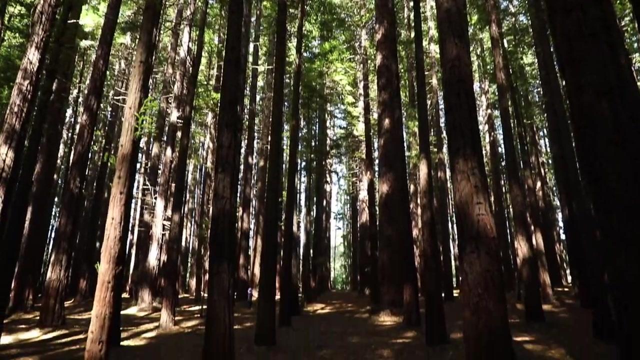 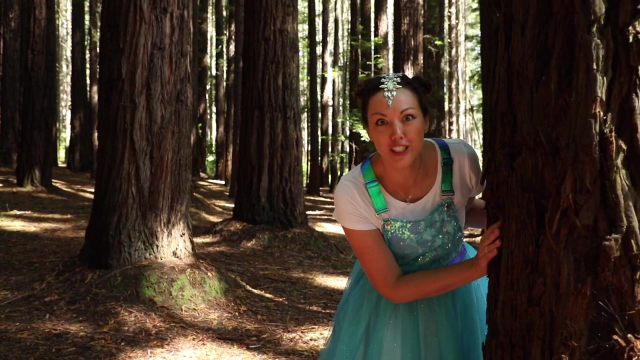 That is really tall. I'm tall, but they're really tall, And they can actually be 1,800 years old. That is so cool. These trees were planted as part of a scientific experiment many years ago. I'm here with some of my friends today, but where are they? It's so tricky to find anyone. 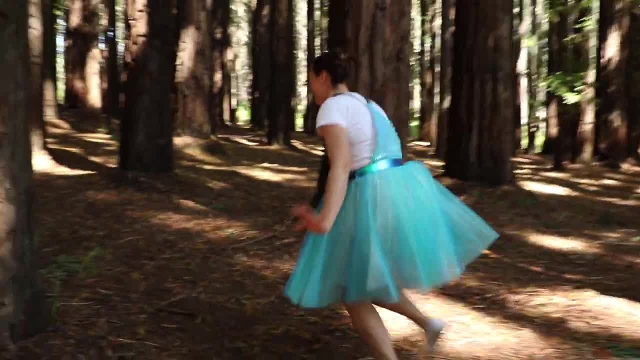 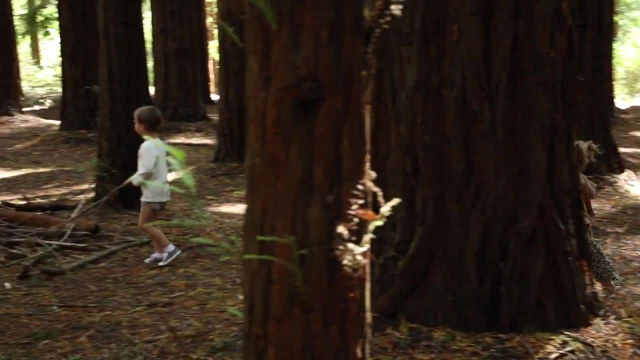 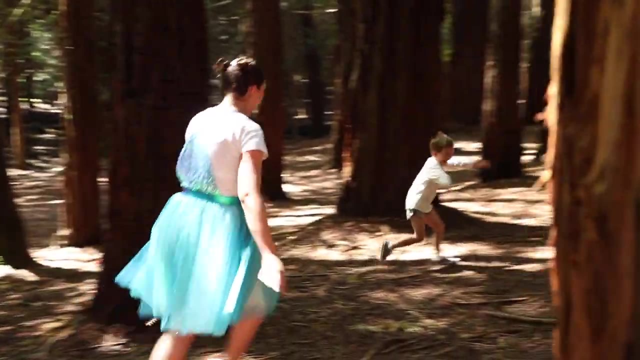 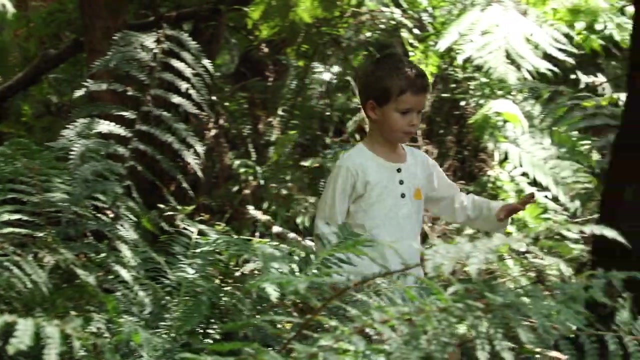 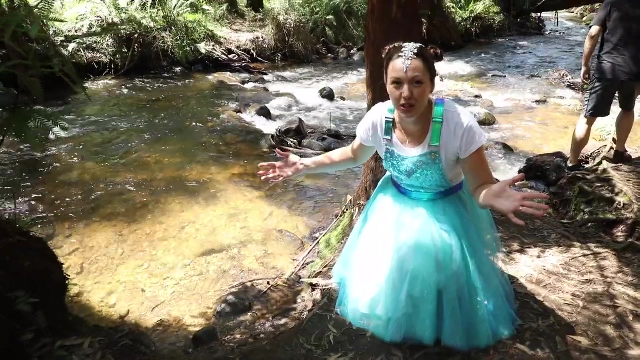 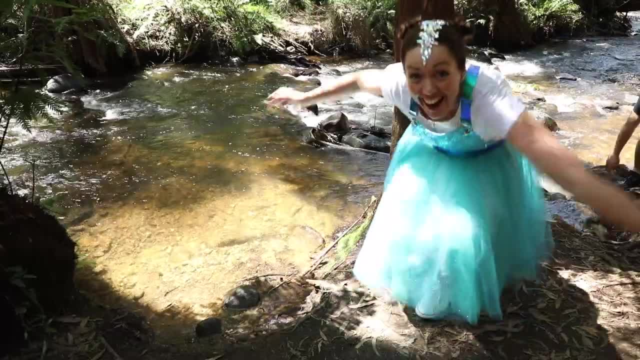 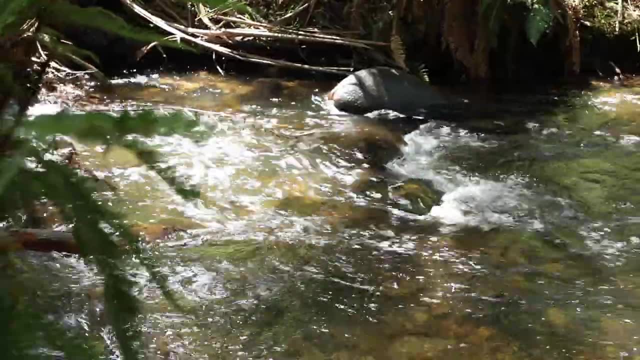 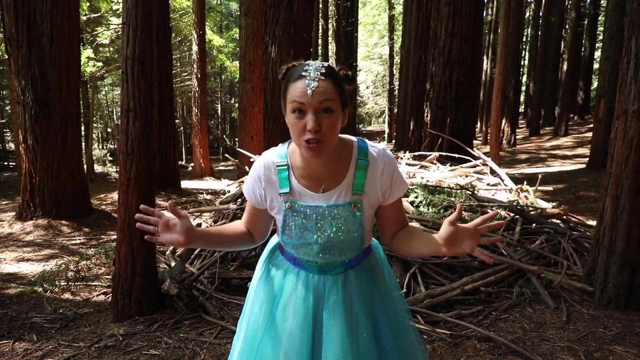 It is gorgeous. Come and have a look. Adding to this mystical and magical feel, you'll find these awesome dragon nest all around the forest. In fact, there's one behind us. now You can add to it if you love to see this feel. 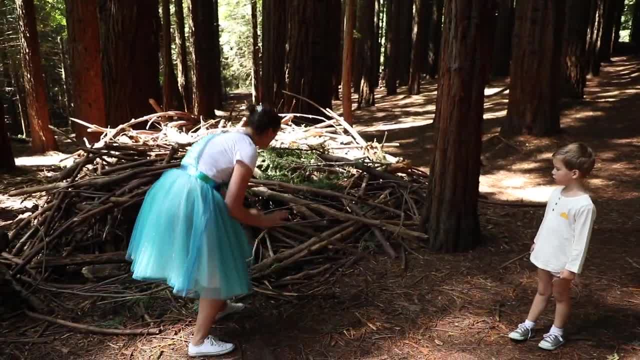 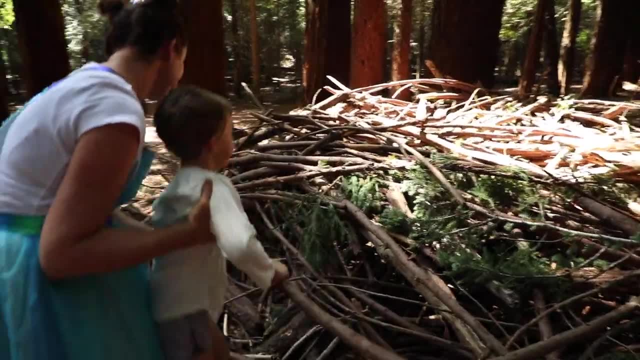 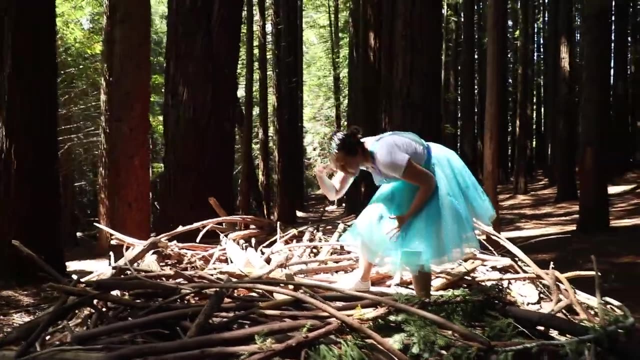 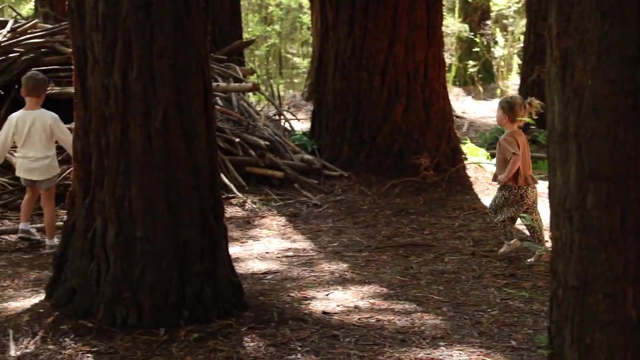 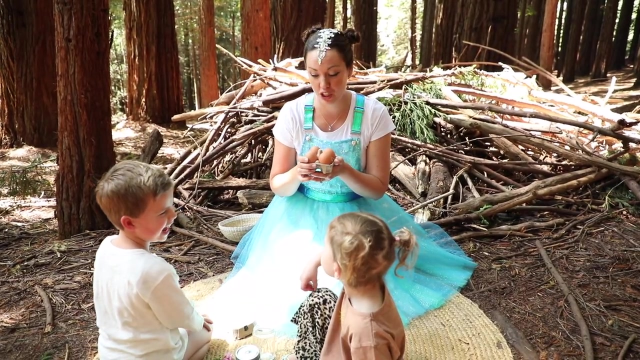 can add to it if you like. Are you ready? We might even find a dragon egg inside the nest. Can you see one? Let's go. One, two, three, four, Oh good, throw, Uh-oh. Speaking of eggs, I'm going to show you a really fun craft activity you can do with just 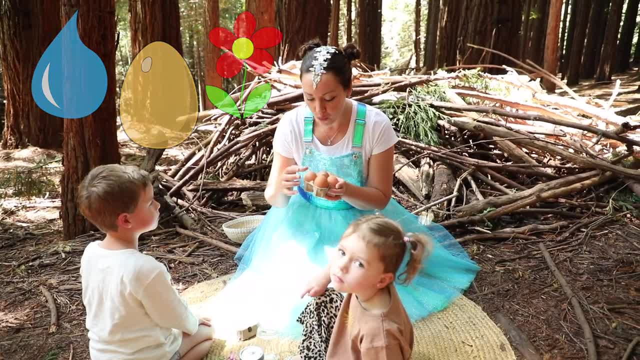 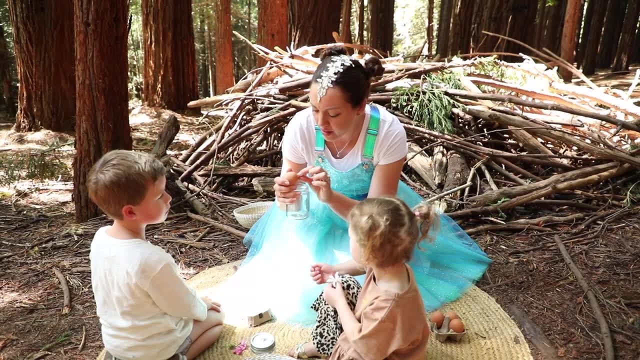 some eggs, water and some flowers. So what we're going to do is crack our eggs a little bit up the top- Very careful, You might need an adult to do this one, Because we just want to hole up the top. empty out our eggs as much as you can. We're going to